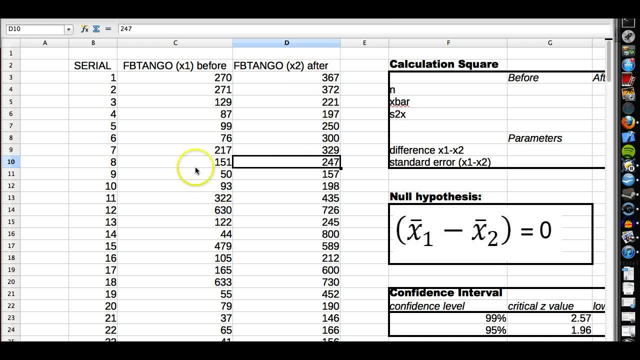 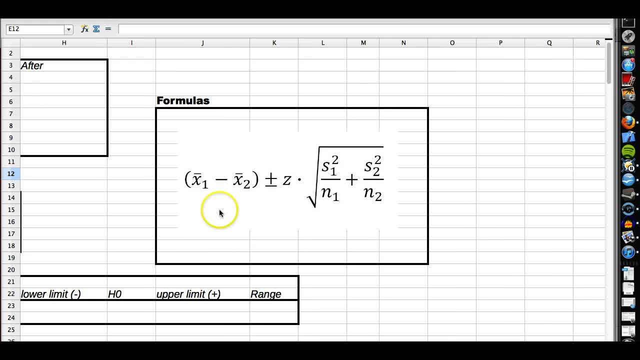 So The mean number of Facebook friends should be larger in this sample than it should be in this sample. So what we're going to have to do is we're going to have to create a confidence interval around the idea that this is not true actually. 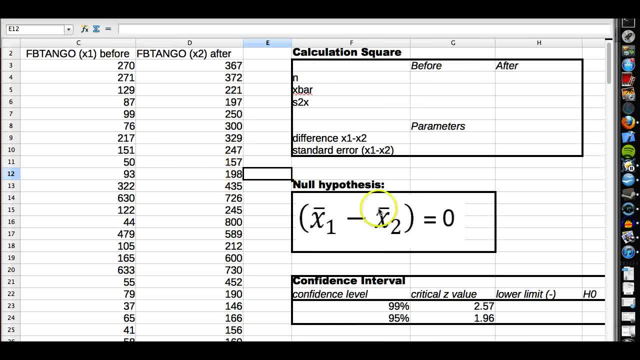 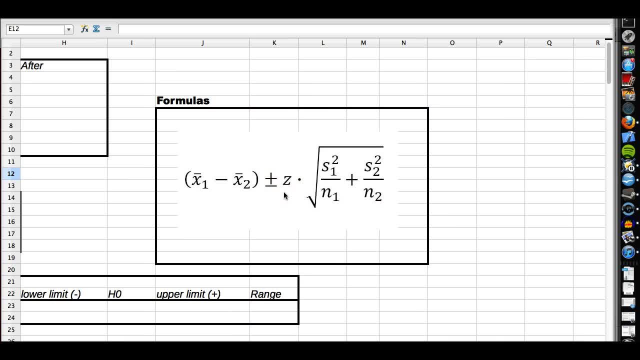 We're testing a null hypothesis, So this will become zero as our null hypothesis, which would mean that the sample means are, in fact, not different from each other. We're going to choose a critical Z value, which means we're using the normal distribution for this in this case. 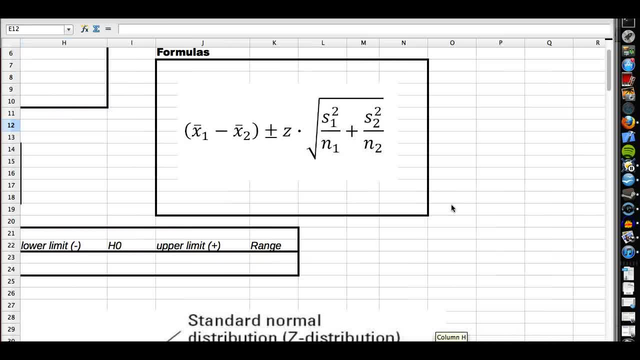 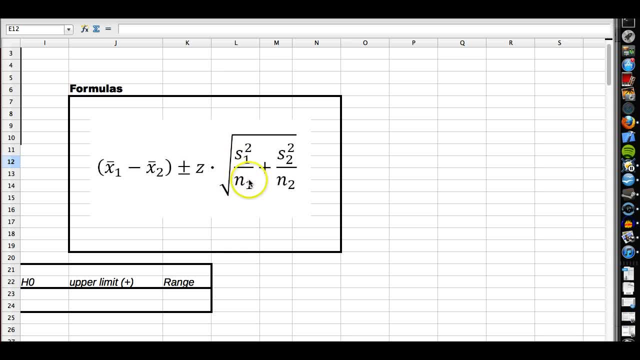 And you can find the critical Z values in a table. It's a two-dimensional, It's a two-sided hypothesis test, because we have plus and minus here And then we're going to multiply all of this by the standard error. Now the standard error here is a pooled standard error, which means we're combining the variation in the first sample and in the second sample and using the sample sizes. 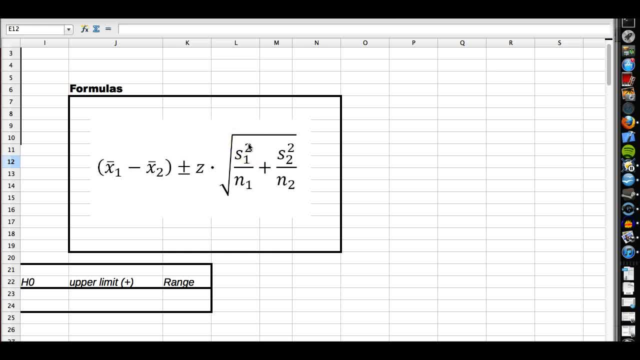 So it's a combined uncertainty, which means we have to make a number of assumptions, And I encourage you to, you know, read up on the literature. I might make a tutorial on it too, But to begin with, for example, we have to assume that we have fairly normally distributed variables and stuff like that. 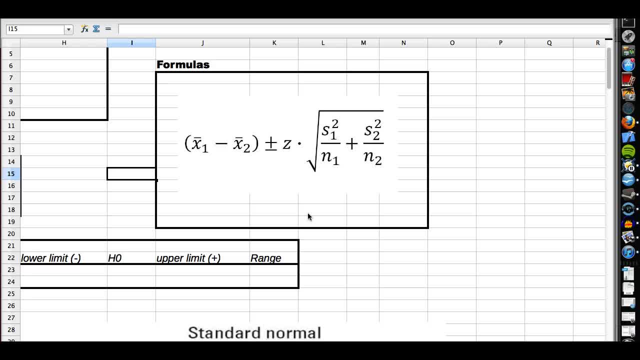 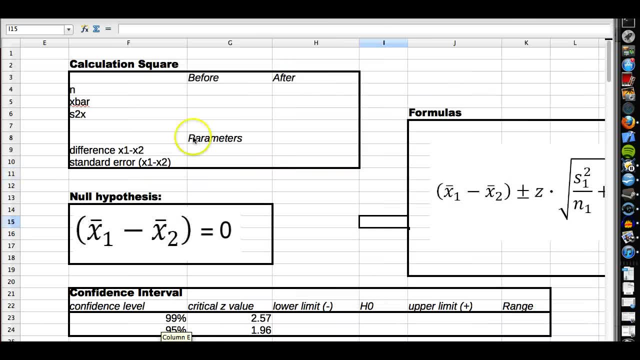 So be careful when you're doing this. Read up on the assumptions that you have to make. So let's start calculating. We're going to need the sample sizes of our two samples, So we're going to start calculating that I write equal to count. 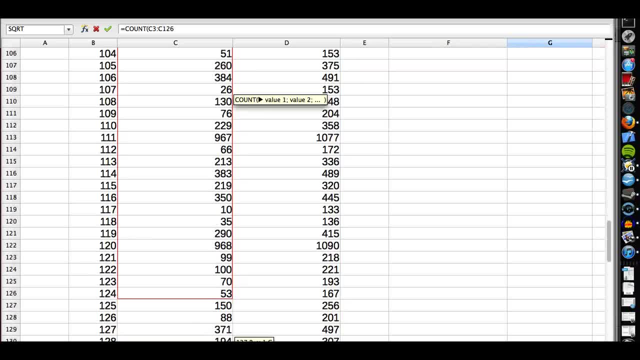 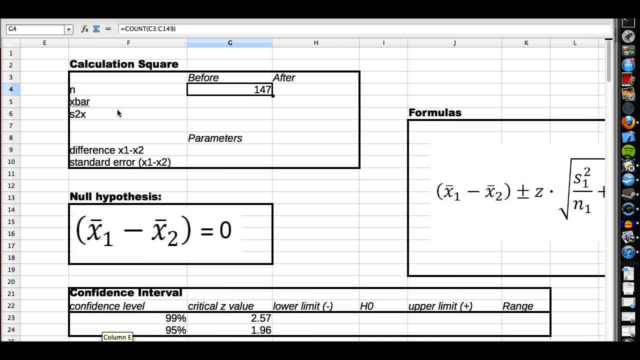 I'm going to count the number of tango dancers in my first sample, And this was before the huge tango festival event. So there I count it and we find that in the first sample we had 147 tango dancers. 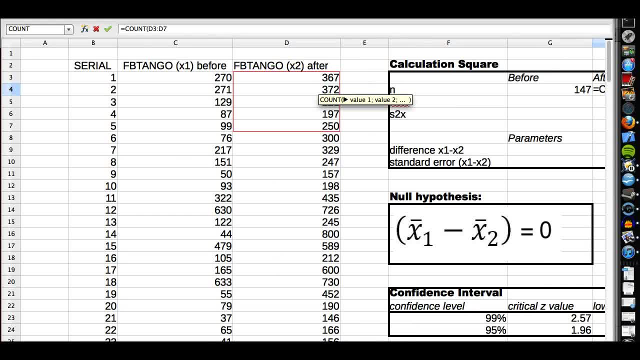 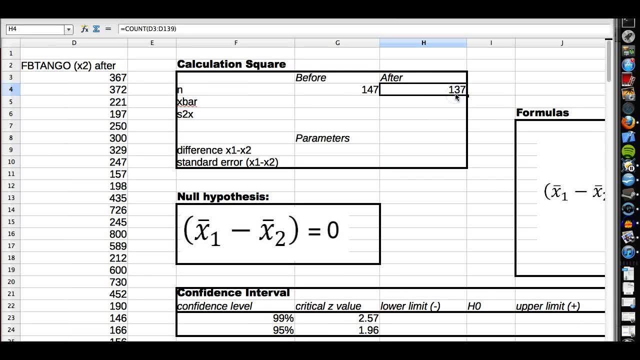 In our second sample, which is The sample after the huge tango dance. I go down here, I select all my data, Close that and I find that I have 137 tango dancers in my second sample. So we have this part of the formula and we have that part of the formula. 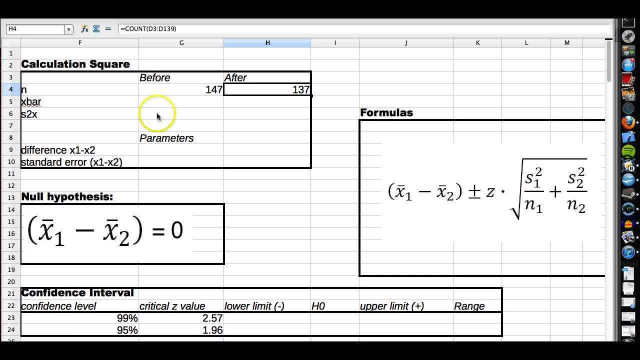 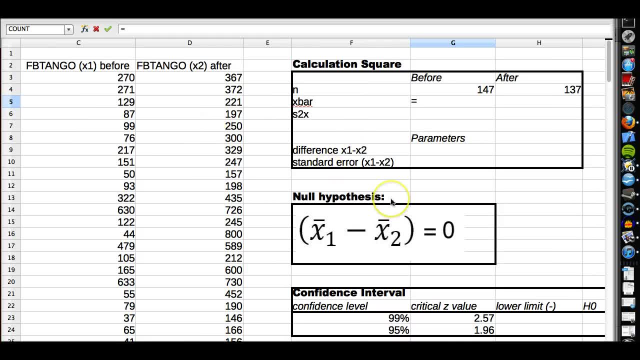 Now we're going to need the variation around the means in our sample And in order to get that, you know we usually calculate the mean first. So we're going to do that. We're going to calculate our estimate first. Average. 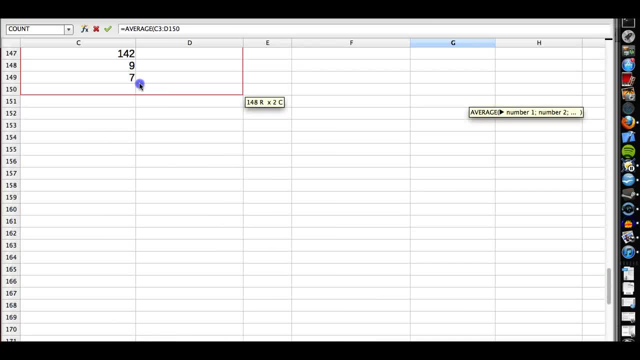 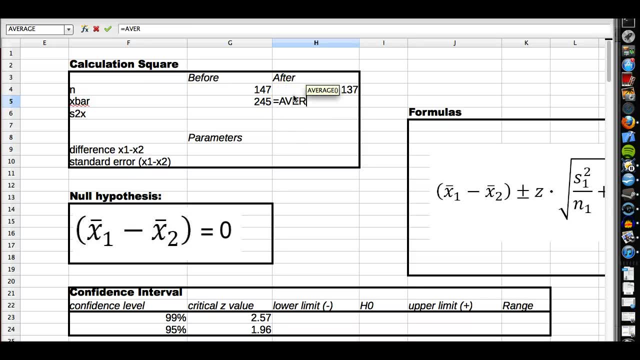 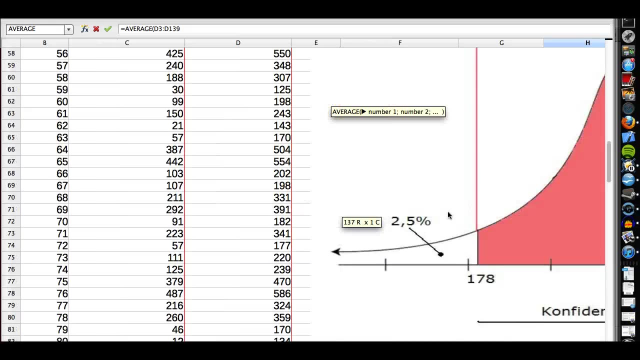 So the average number of Facebook friends they had before Or that tango dance festival of awesomeness, was 245 Facebook friends on average After the dance Huge festival they had. and this is exciting. Well, it's more exciting for you because I know the answer, because I created the data. 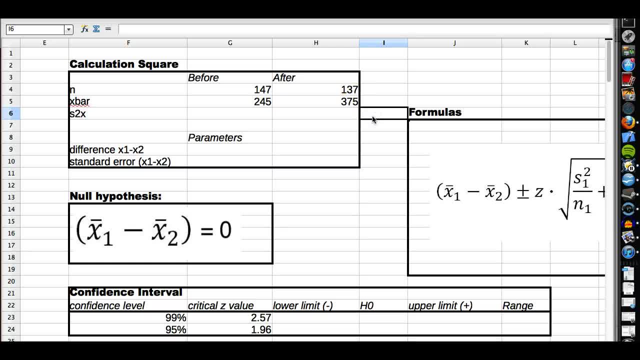 It's 375.. So you might say, okay, hey, look, there's a difference. They had more Facebook friends after the festival than they had before. Enough said you know, end of story. That's not true. This would only be true if we had. 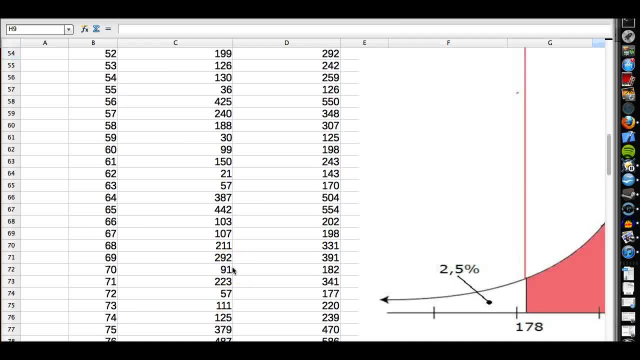 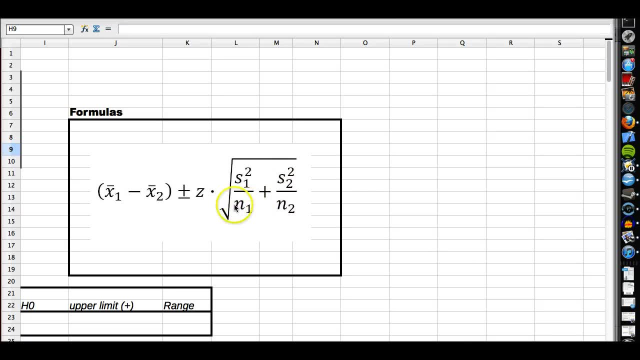 If we had asked all the tango dancers that participated in the festival. but we haven't. We have samples, So we have to take our uncertainty into account, And that's what the standard error is all about. We're going to need 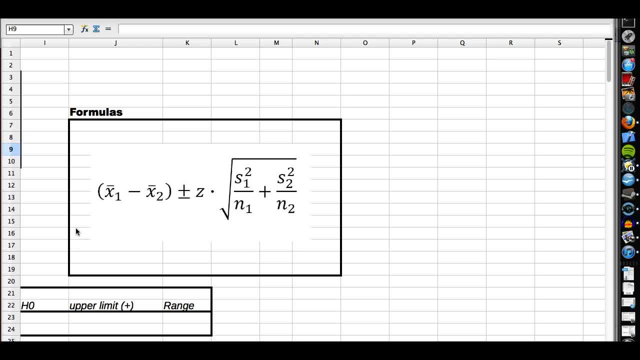 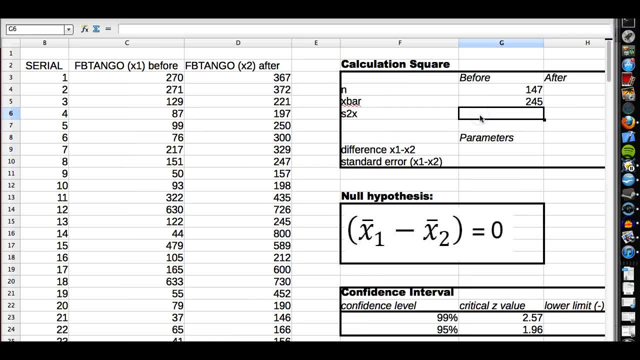 That's why we calculated the sample sizes. You know that matters. How many people did we ask? And the variation around our means, because that says something about how uncertain we can be about the guesses. How much does it vary? So we're going to calculate that by var V-A-R for the variation for our first sample. 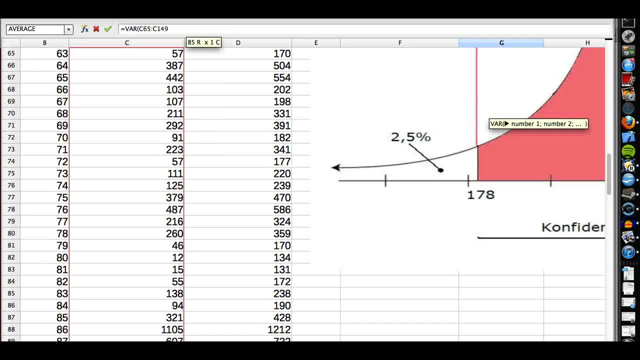 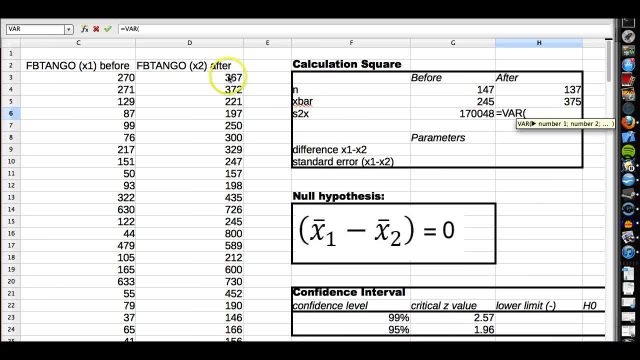 Go down up. I missed it. I'm going to have to do it again There. I select my entire data set like that And I get a variation. I'm going to do this for the second sample as well. Var. 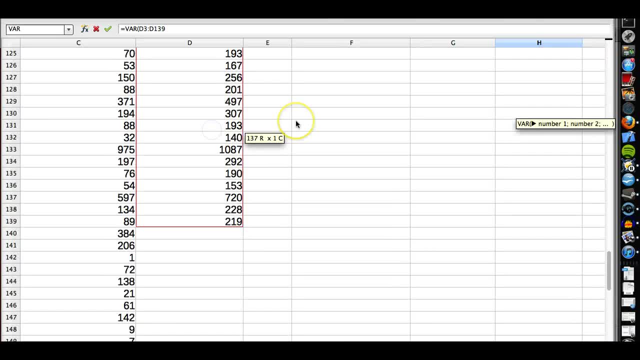 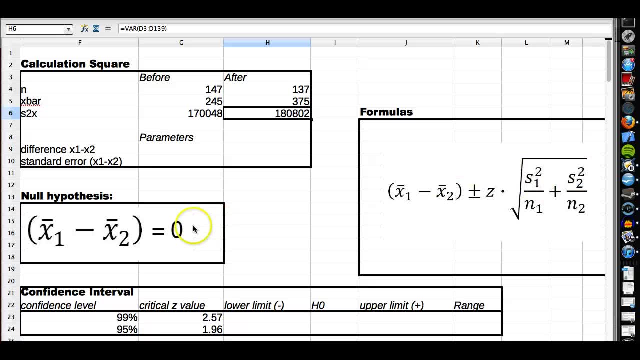 I go down here, I select my entire data set. There we go, Close that And I get a second variation. So now we have our ends, We have our variations, We have our critical Z values, because I looked them up in a table for you, remember. 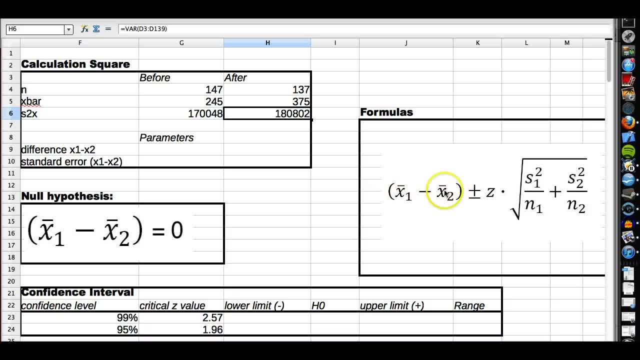 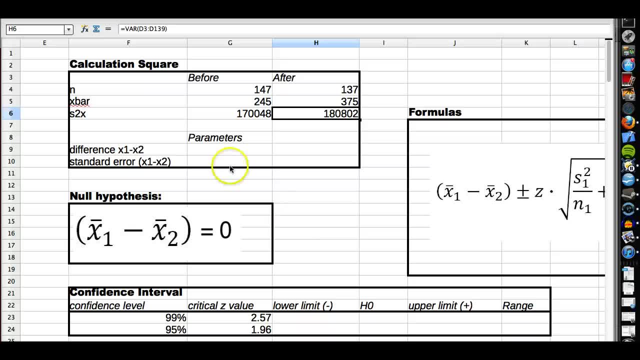 And we have the null hypothesis, which is that this difference here is going to be equal to zero. So we can actually start calculating Our confidence intervals. But to make this easier, we're going to calculate the standard error here, in its own area, so to speak. 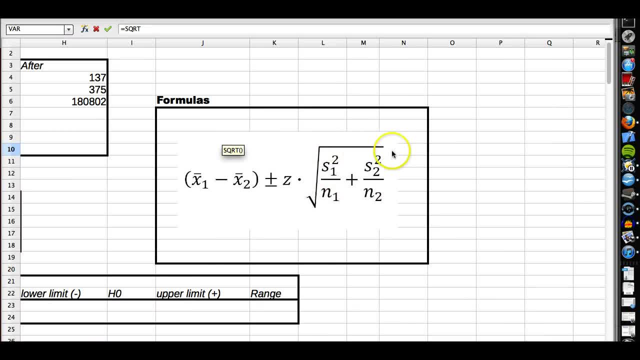 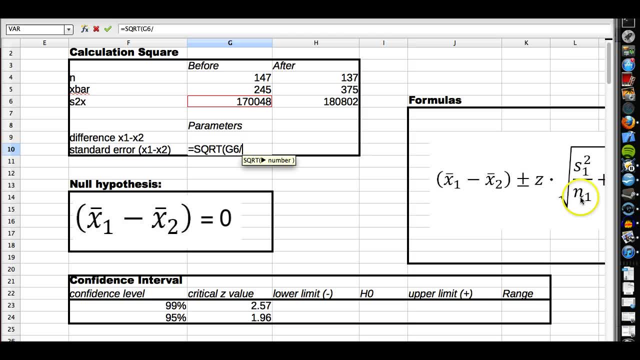 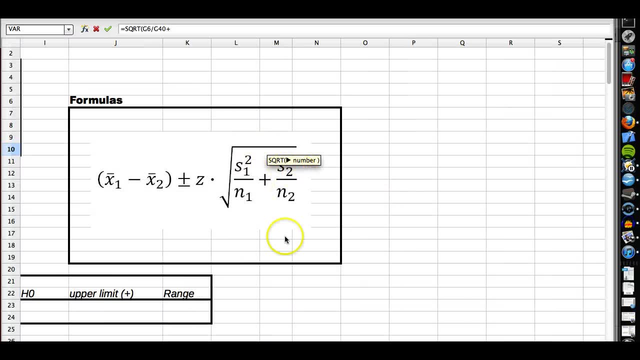 So square roots. See here Square roots. I'm going to take the variation in my first sample Right there, Divided by the number of people. in my first sample I'm going to add the variation. You can see it there. 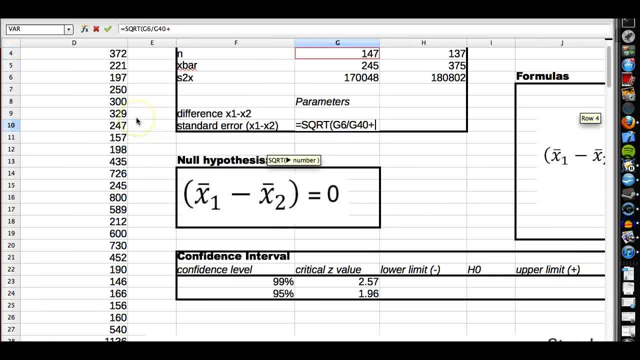 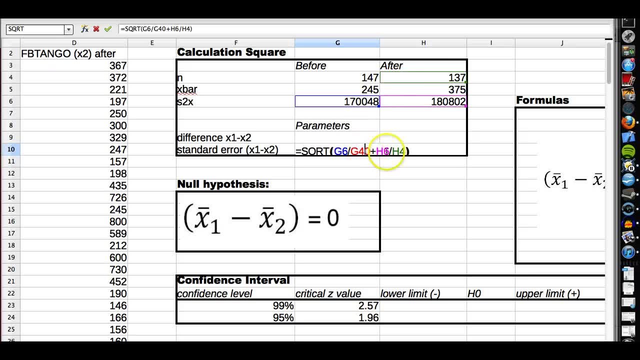 The variation in my second sample divided by the number of people in my second. So I choose my variation there, Divided by the number of people. Close that parenthesis. Oops, And I did some kind of mistake here. All right, This is. 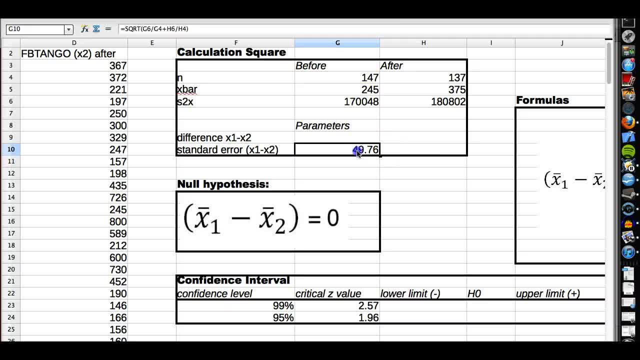 I'm sorry about that, guys. There I'll calculate it again so it's clear: Square roots of the variation in my first sample divided by the number of people in my first sample, Plus the variation in my second sample divided by the number of people in my second sample. 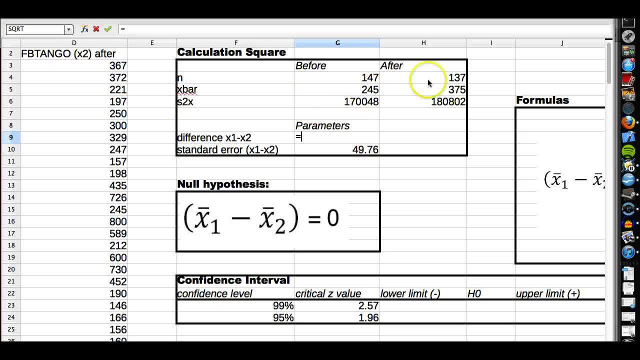 And there we get our standard error And the difference between these two is our test variable. you could say It's not really the test variable, but it's the difference that we are going to be comparing to our confidence interval. So I'm going to take x1 here, minus x2.. 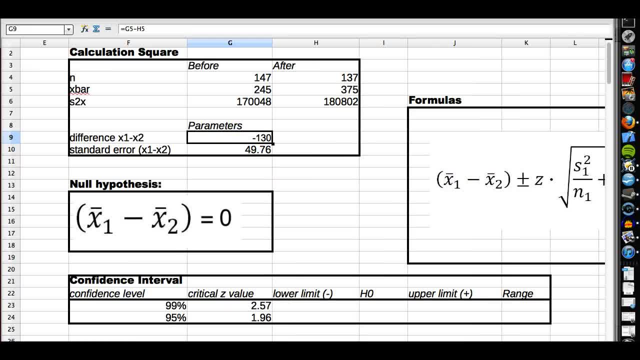 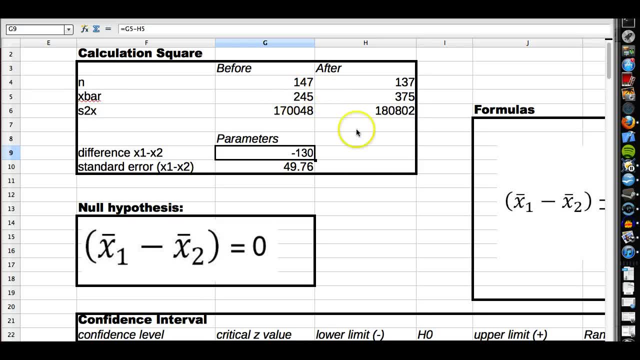 You see it there: x1 minus x2.. And I get minus 130.. Now it's time to stop and think for a second. You might be questioning this, because it says minus there, And you can see that this number is larger than this one. 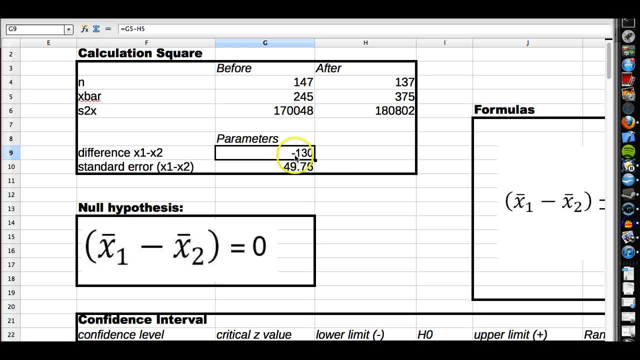 So you say, but they had more friends after the dance. Why are we getting minus here? What does that mean? Well, it really doesn't mean anything right now, because we're doing a two-sided test, Because we're testing around a confidence interval with a positive side and a negative side. 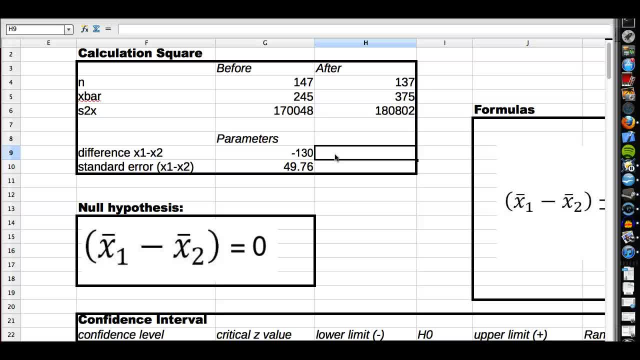 So we're just looking at the absolute difference. you know in absolute terms. We're not saying in which direction it's going. I might as well do this, I could do this and get 130.. So it really doesn't matter if you have minus or plus there. for now, 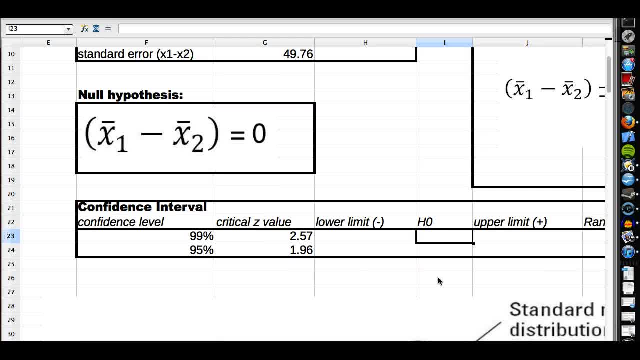 So bear that in mind And we're actually ready to start calculating our confidence intervals, which we're going to be comparing to this distance here. So H0, my null hypothesis is that that's a center point 0. There's no difference between the samples. 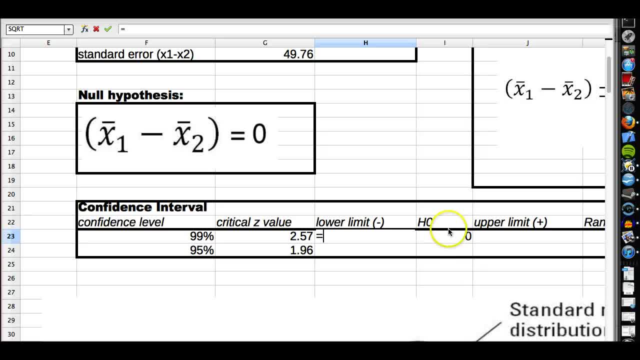 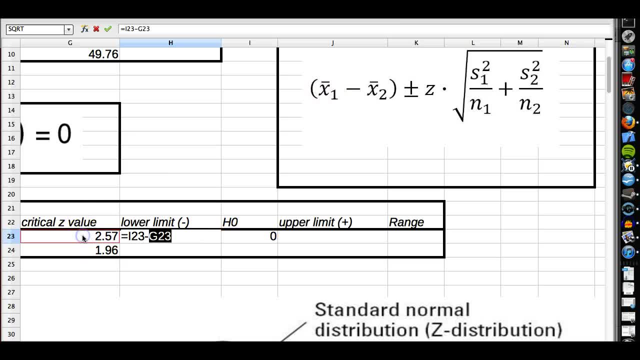 And the lower limit on the confidence interval around. that idea is my difference, which is this part of the formula minus, because we're working with a lower limit, our critical Z value multiplied by the standard error which I have there, And I get my lower limit of minus 128.. 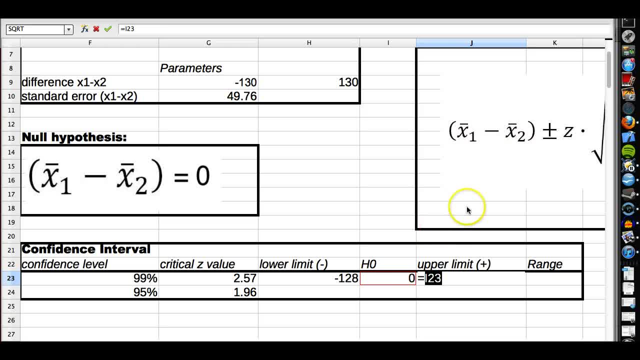 The upper limit, meanwhile, is going to be 0,. so the formula plus a critical Z value- and this is at 99% confidence level, just so you know- okay, multiplied by the standard error, and I get my upper limit, which is 128. 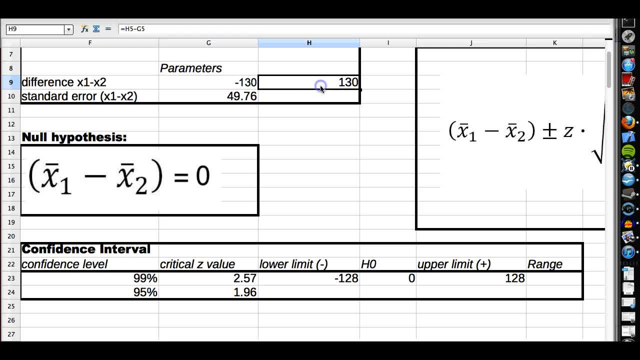 Now what I do now is I take a look at this difference here: 130 in absolute terms. Is that within our interval? No, it is not. It is larger than 128.. And in illustrative terms, this is what's happening here. 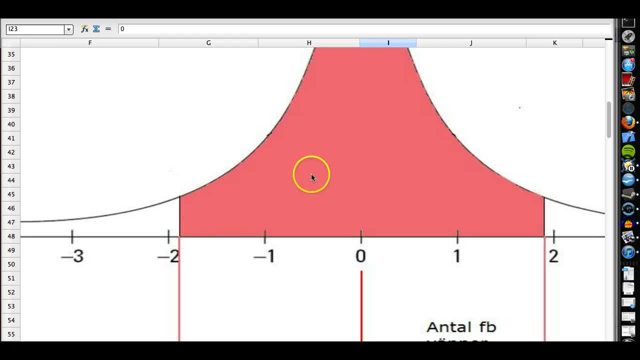 We have a confidence interval. This is done for 95% confidence level, but it's the same principle. We have a confidence interval here. We have our critical Z values and in this case it's 2.57, so 2.57, somewhere around there. 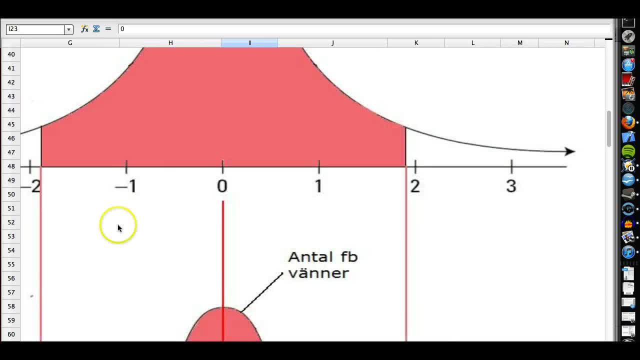 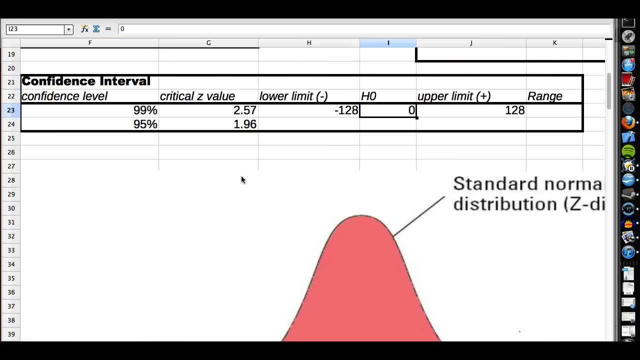 We've translated this into number of Facebook friends, so it's going to be minus 128 there and plus 128 there, And we're comparing that to the real difference that we found between our samples, so we can find that that is located in our tails, right. 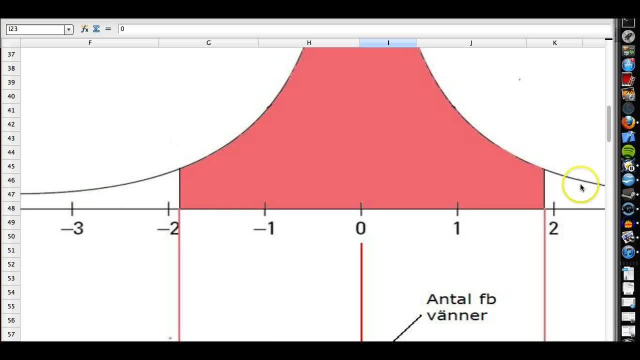 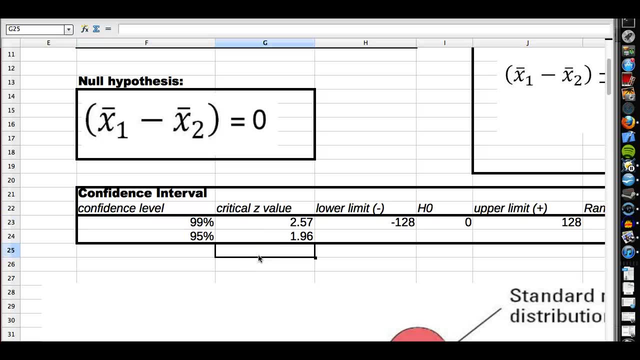 Right, So our sample difference is located in our tails. And what does that mean? Well, when we have a confidence level, what we're saying is that if I conducted this sample 100 times, in 99 of these cases I would get a mean that varied randomly between these two values. 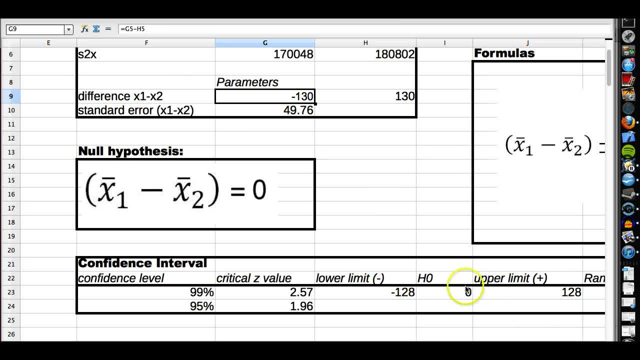 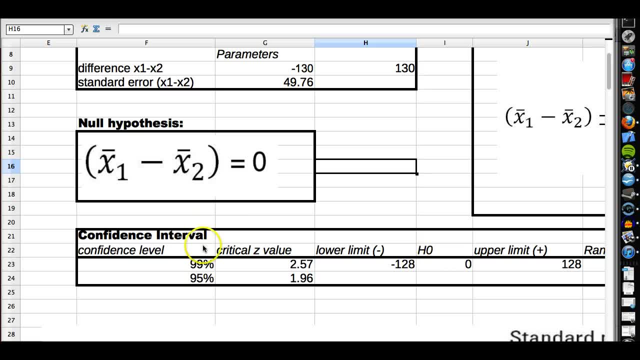 Now that's not what I'm getting. I'm getting a larger, different mean outside of this interval. That could either be because of the freak chance- which is 1 out of 100, that I'm just unlucky and I'm getting an extreme sample that is outside of our interval, or it could mean 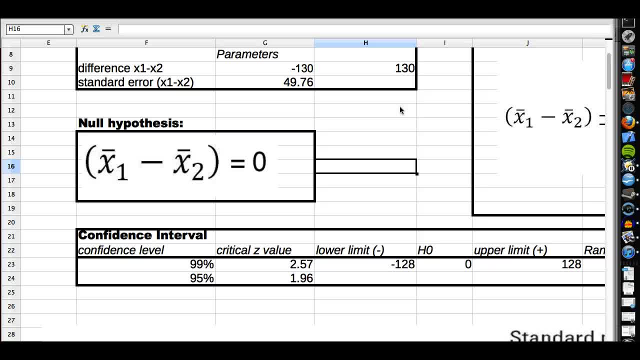 that a real change has occurred, And that's what we mean by statistical significance. We're saying that the chance is very, very low that this change is just due to randomness. So we're saying that a statistical change has actually occurred. Now we're going to do this for a 95% confidence level too, just to practice. 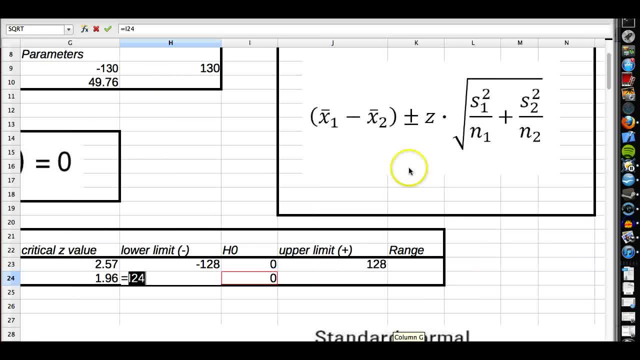 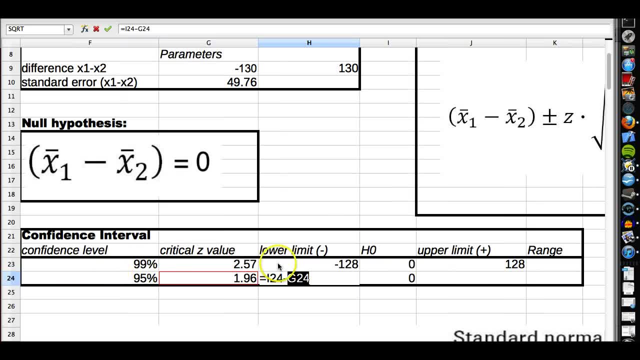 So same null hypothesis. I select my distance, which is this part of the formula minus, because I'm working with a lower limit, My critical value, which has changed because I changed my confidence level, multiplied by the value of my confidence level, which is 0.. 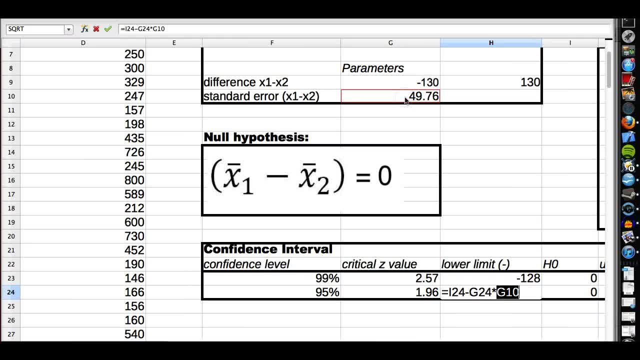 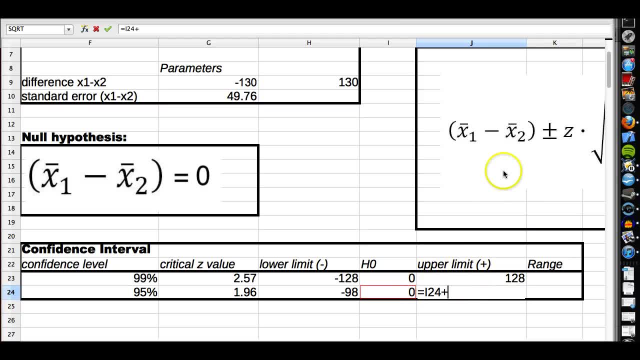 Multiply by the standard error, which is there. So I choose my standard error there and I get a lower limit. Same thing for the upper limit, but this time I'm working in the upper limit. so it's plus My critical z value, multiplied by the standard error and I get my upper limit. 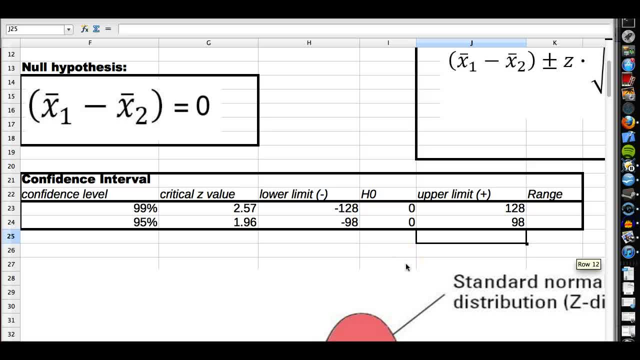 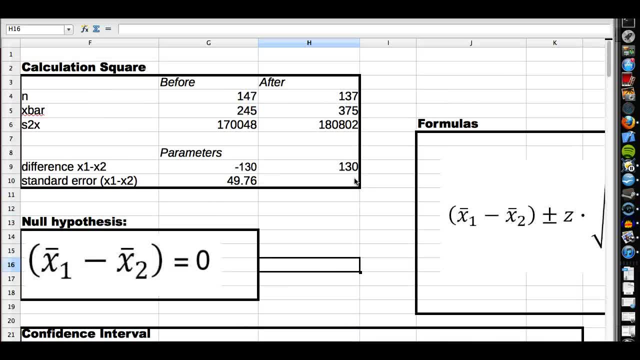 And you know it's still a significant change, statistically significant. So our null hypothesis is refuted in both cases And basically that's how you can use confidence intervals to test a hypothesis And it's closely Relate to the stuff that we're going to be doing in the future tutorials. 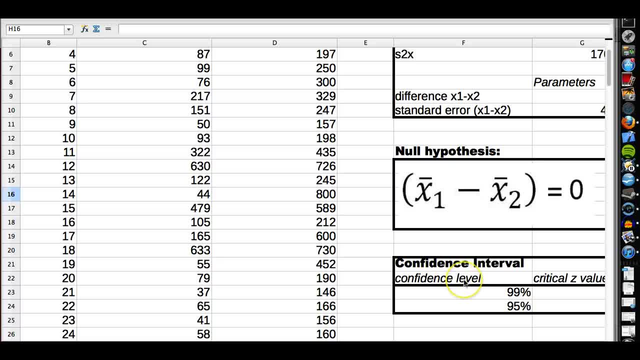 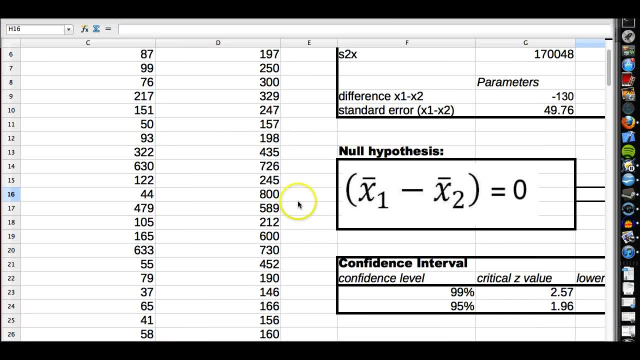 So consider this tutorial when we're working on the future ones, and you'll understand the principles behind the scenes, so to speak, when we're working. So have some fun with this, Try changing the values and checking what happens. I hope you have a really great day and good luck with this stuff, guys. Bye-bye.